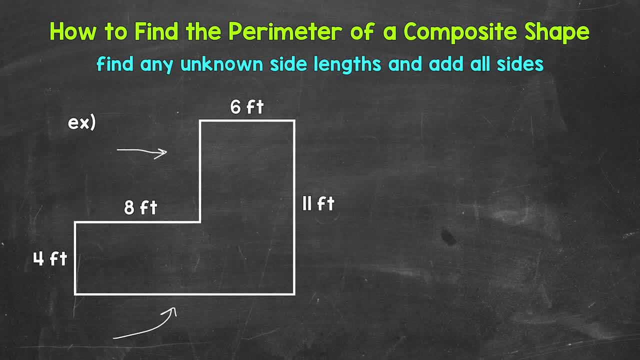 what we do not know. For example, we know that this vertical side right here measures 11 feet. We can use that to figure out what this missing side equals. We know that this is 4 feet plus. what will give us that 11 feet? Those two vertical sides need to equal 11 feet. Well, 4 feet plus. 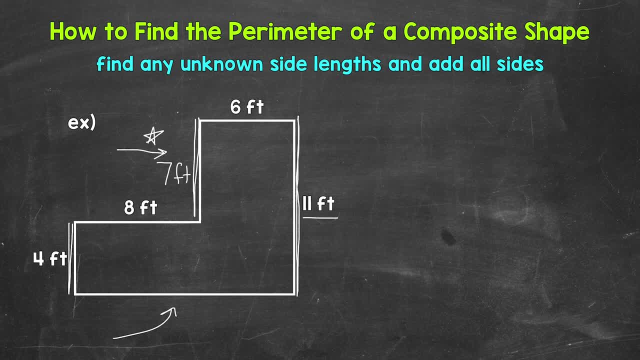 7 feet equals 11 feet. so that missing side length equals 7 feet, because again we have 4 feet plus 7 feet gives us 11 feet. We can use that to figure out what this missing side equals, That 11 feet. Now we can figure out this missing side length right here. so this horizontal side. 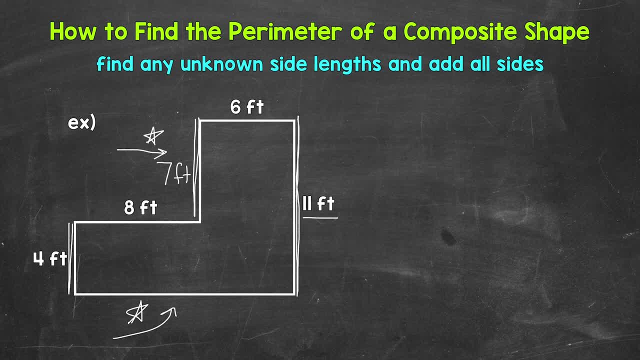 Again, we need to use what we know, what we are given, to figure out that missing side length. So let's use these two horizontal lines Right here. we have 8 feet and we have 6 feet. Those two sides are going to equal that missing side length. So we have 8 feet plus 6 feet. 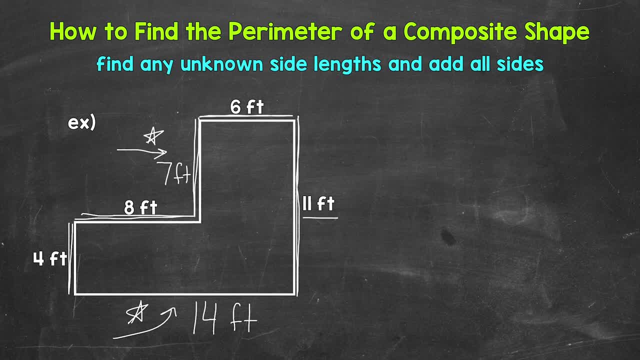 gives us 14 feet. So that missing side length measures 14 feet. Now we can add all of the sides in order to find the perimeter. So perimeter equals, and I will start with 6 feet here. so 6 plus 11.. And I'm going to cross off the sides as I go around. That way I make sure I don't forget. 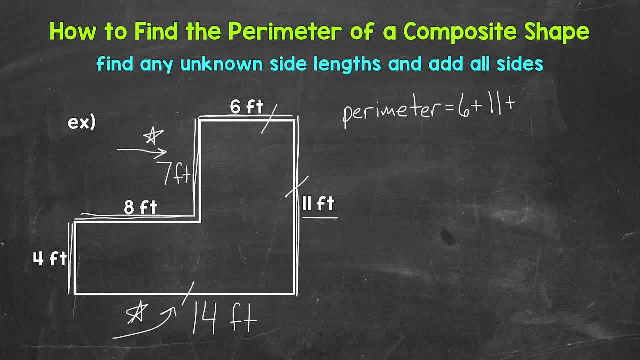 anything or count anything. So I'm going to cross off the sides as I go around. So I'm going to cross off the sides as I go around. That way I make sure I don't forget anything or count anything. So next we have 14 plus 4 plus 8 plus 7.. So 6 plus 11 is 17,. plus 14 is 31,, plus 4 is 35,, plus 8 is 43,. 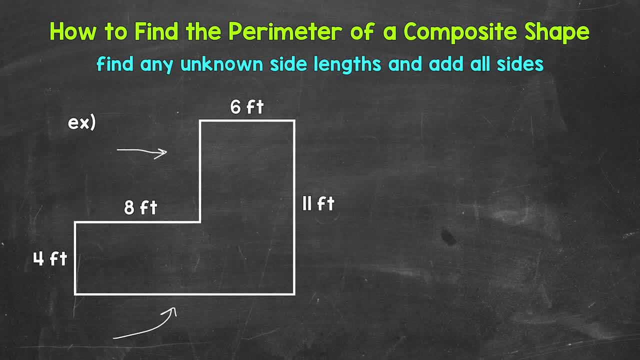 what we do not know. For example, we know that this vertical side right here measures 11 feet. We can use that to figure out what this missing side equals. We know that this is 4 feet plus. what will give us that 11 feet? Those two vertical sides need to equal 11 feet. Well, 4 feet plus. 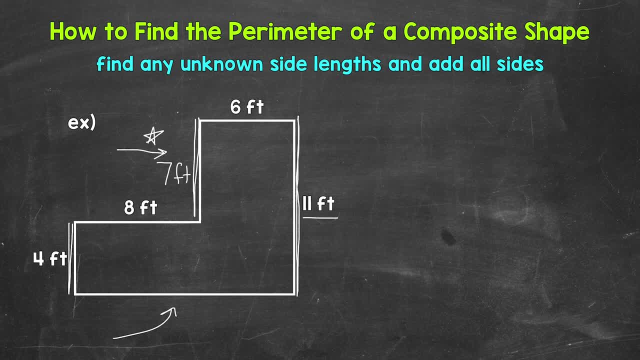 7 feet equals 11 feet. so that missing side length equals 7 feet, because again we have 4 feet plus 7 feet gives us 11 feet. We can use that to figure out what this missing side equals, That 11 feet. Now we can figure out this missing side length right here. so this horizontal side. 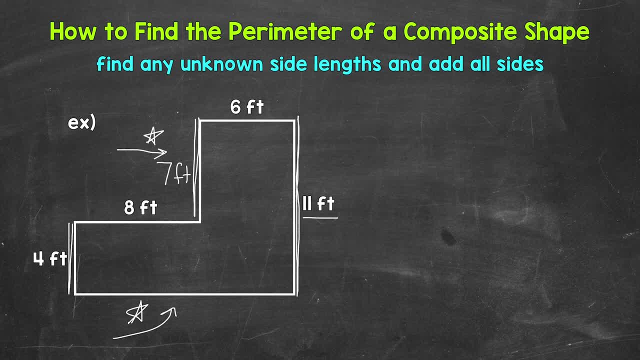 Again, we need to use what we know, what we are given, to figure out that missing side length. So let's use these two horizontal lines Right here. we have 8 feet and we have 6 feet. Those two sides are going to equal that missing side length. So we have 8 feet plus 6 feet. 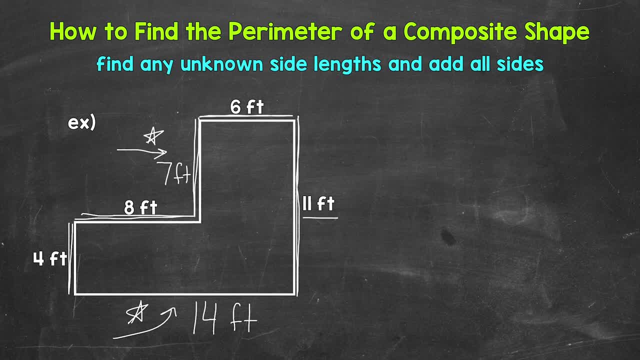 gives us 14 feet. So that missing side length measures 14 feet. Now we can add all of the sides in order to find the perimeter. So perimeter equals, and I will start with 6 feet here. so 6 plus 11.. And I'm going to cross off the sides as I go around. That way I make sure I don't forget. 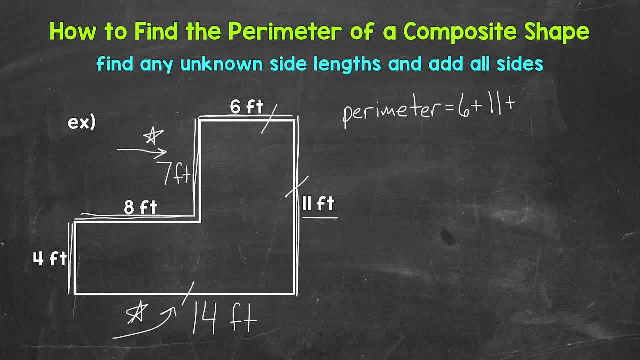 anything or count anything. So I'm going to cross off the sides as I go around. So I'm going to cross off the sides as I go around. That way I make sure I don't forget anything or count anything. So next we have 14 plus 4 plus 8 plus 7.. So 6 plus 11 is 17,. plus 14 is 31,, plus 4 is 35,, plus 8 is 43,. 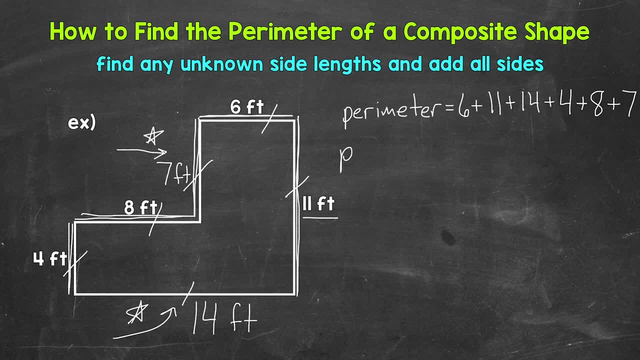 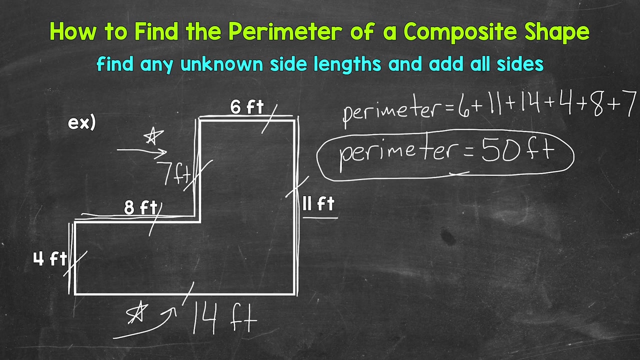 plus 7 is 15.. So the perimeter equals 50 feet. So there you have it. There's how to find the perimeter of a composite shape. If you have any unknown side lengths, start there. So find any unknown side lengths first. Once you have those, add all of the sides and you have the perimeter. 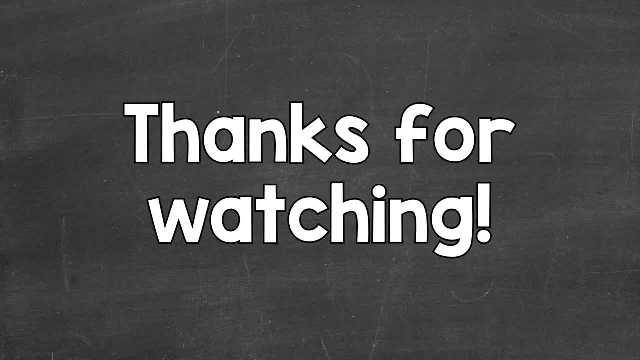 I hope that helped. Thanks so much for watching. Until next time, peace. 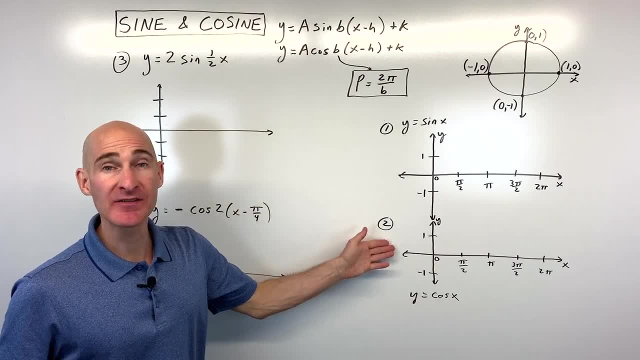 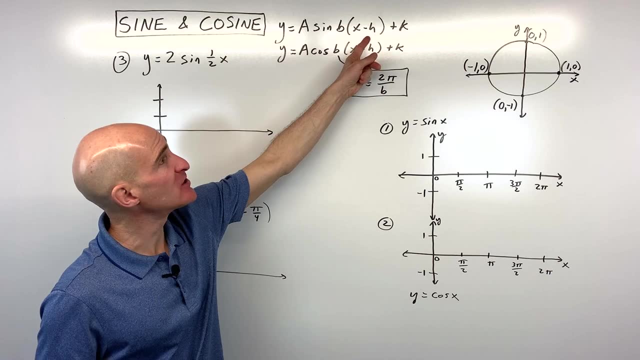 In this video, you're going to learn how to graph the sine and cosine graphs, as well as graphing sine and cosine when they're transformed. We're going to be working with this general formula right here: where h is the horizontal shift, k is the vertical shift, b is related to 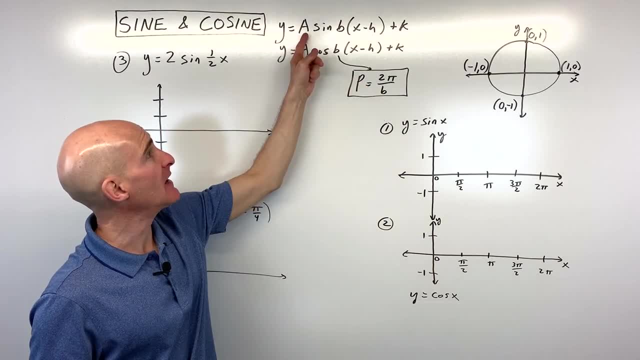 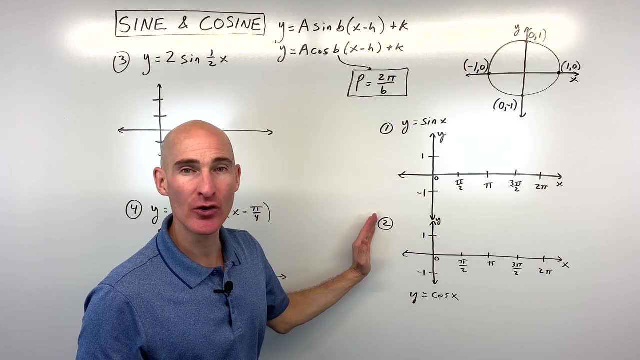 the period through this formula, 2 pi divided by b and then a is going to be our amplitude or our vertical stretch, or compress. So let's start off by talking about how do you graph the basic sine and cosine graph. Well, if you go to the unit circle, which you probably already learned about, 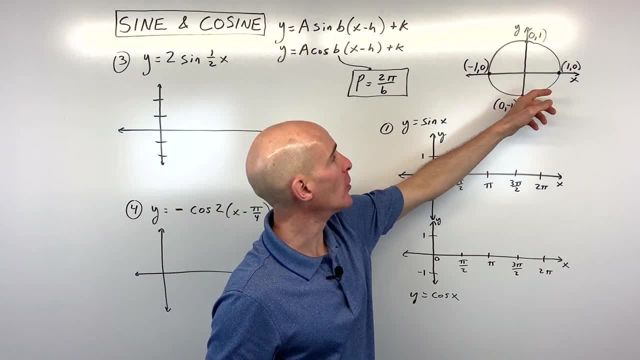 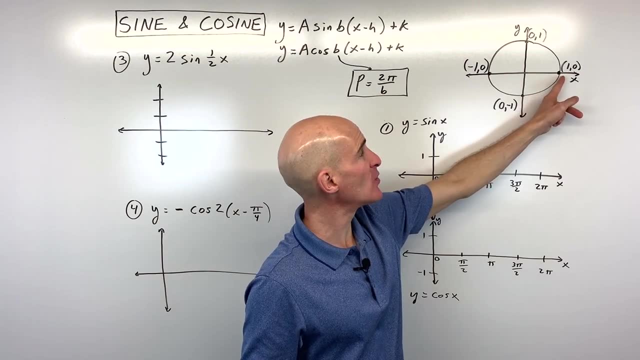 previously, if not, check out my mastering the unit circle video. When we think about the unit circle, when we're talking about sine, what we do is we go to the angle- for example, zero radians- and we say what's the sine of zero radians? Well, it's going to be the y coordinate, So you can see. 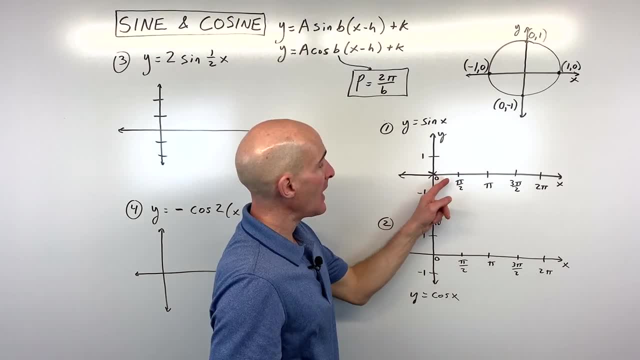 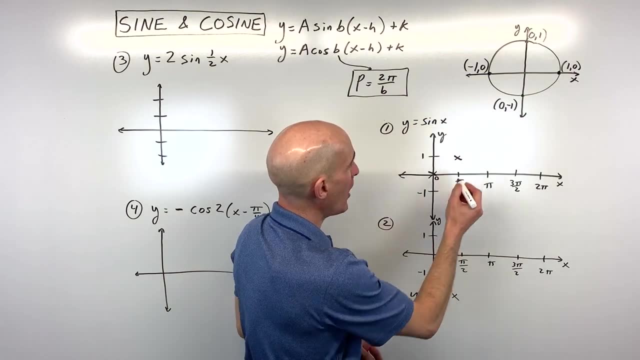 at zero, sine is going to be equal to zero. At pi over 2 or 90 degrees, you can see that the sine, the y value, is going to be 1.. So at pi over 2, let's put a point at 1.. And then at pi 180 degrees. 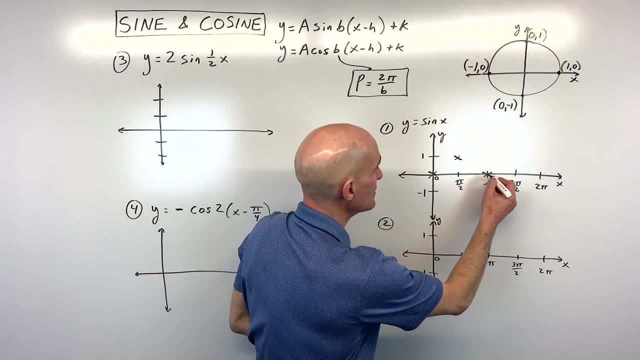 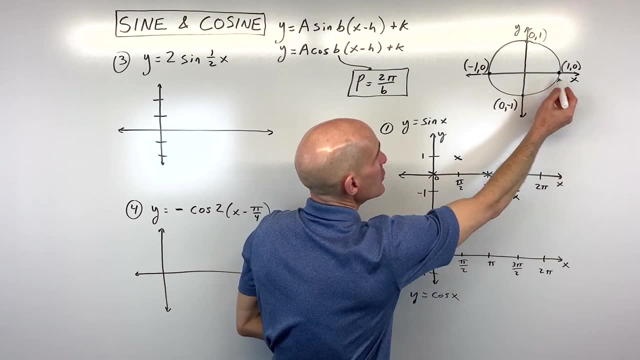 you can see that the y value is going to be zero. So that's going to be right there. And then, at 3 pi over 2, which is right here- you can see the sine value is negative 1.. And then, at 2 pi, you're back to zero. And what happens is that this graph just